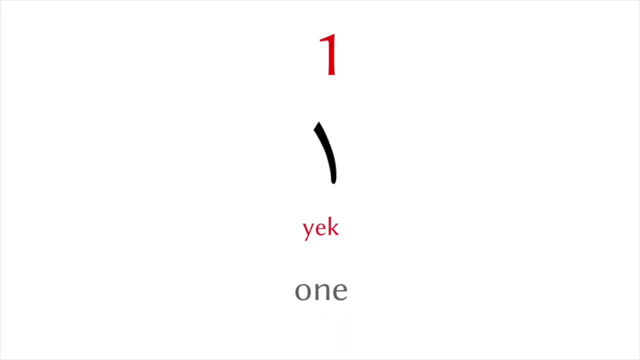 one yik two do three, vse, four, four, five, panj six, six, six, six seven haft haft haft eight, eight, nine, ten, eleven, twelve, thirteen, fourteen, fourteen, fifteen, fifteen, sixteen, eighteen, nineteen, twenty, twenty, twelve, nine, twelve, three, eleven short four, three, four, five, six. 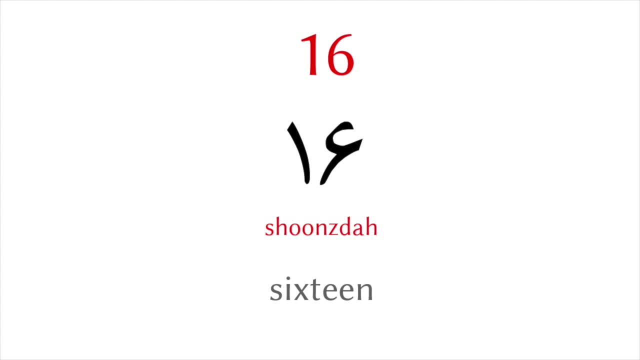 seven, seven, twelve, nine, eleven, fifteen, sixteen, eleven a seven eleven eleven. HEFDAH, EIGHTEEN, HESHDAH, NINETEEN, NUZDAH, TWENTY BEAST, TWENTY-ONE, BISTOYEK, BISTOYEK. 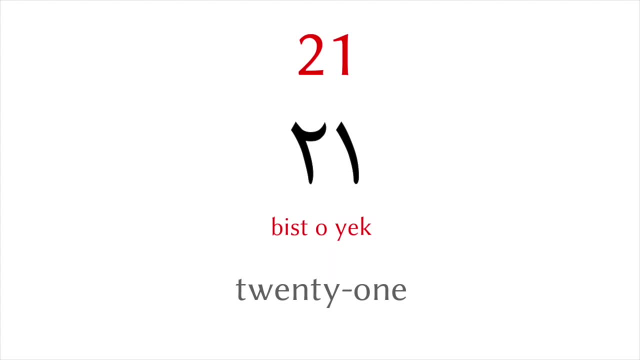 BISTOYEK TWENTY-TWO, BISTODO, BISTODO, BISTODO. TWENTY-THREE BISTOSE, BISTOSE, BISTOSE, BISTOSE, BISTOSE, BISTOSE, BISTOSE TWENTY-FOUR. 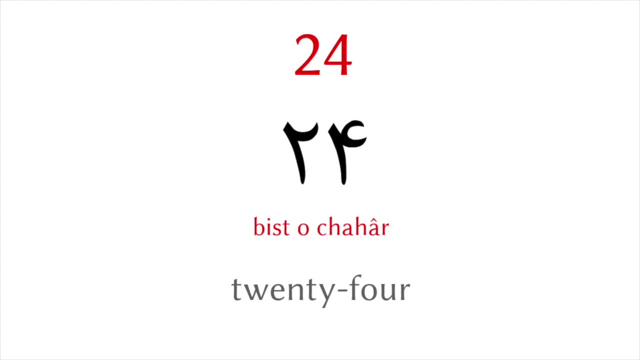 TWENTY-FOUR BISTOCHAHAR, BISTOCHAHAR, BISTOCHAHAR, BISTOCHAHAR, POUT, POUT. TWENTY-FIVE, BISTOCHAHAR, TELLING BISTOCHAHAR. 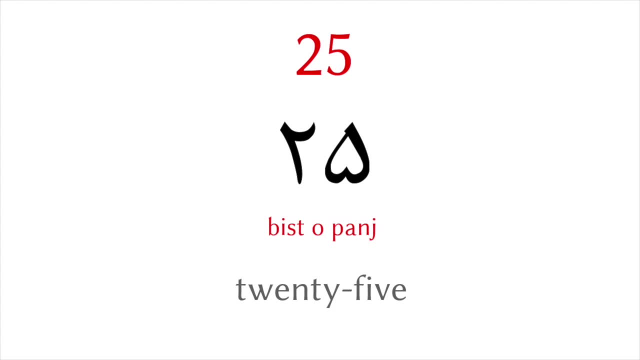 BISTOCHAHAR, BISTOCHAHAR, BISTOPANJ, BISOPANJ, TWENTY-SIX, TWENTY-SIX, Mr Sheesh, Mr Sheesh, Mr Sheesh, Mr Haft, Mr Haft. 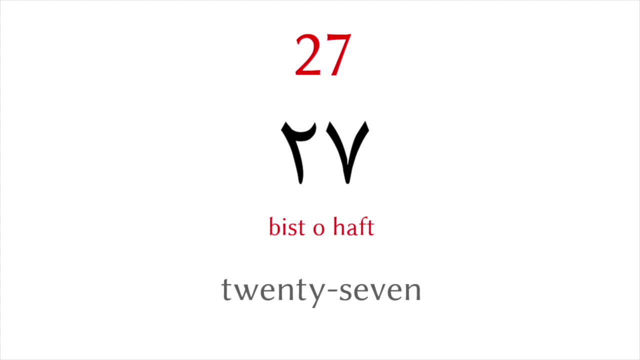 Mr Haft, 28 Mr Hushed, Mr Hushed, Mr Hushed, 29 Mr No, Mr No, Pistón, no. Thirty Sí, Sí, Sí, Thirty-one Sí, o yek. 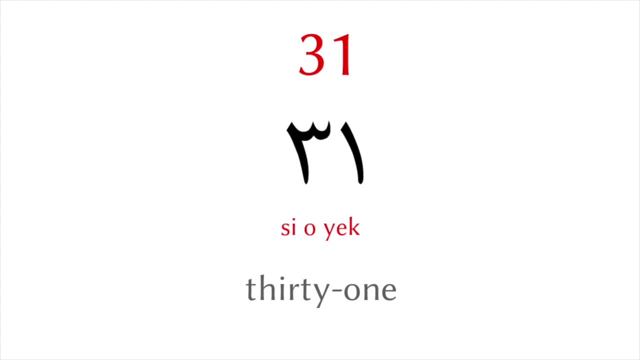 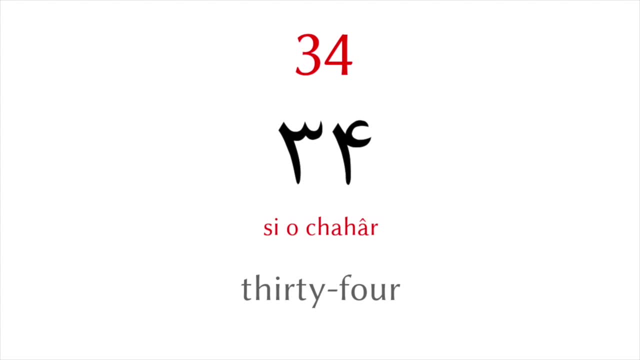 Thirty-four, Sí o chahar, Sí o chahar, Sí o chahar. Thirty-five, Sí o panj, Sí o panj, Sí o panj. Thirty-six, Sí o sés. 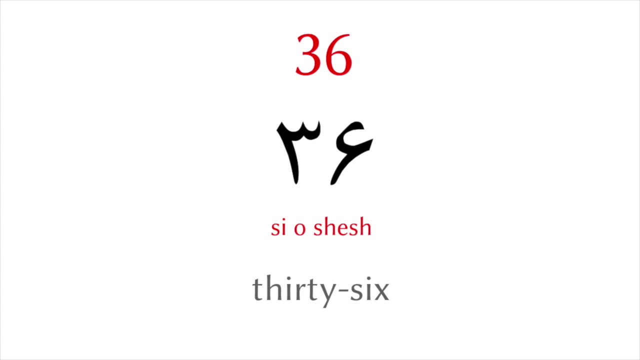 Sí o sés, Sí o sés. Thirty-seven, See your haft. See your haft. See your haft. Thirty-eight, See your hast. See your hast. See your hast. Thirty-nine, See your no, See your no. See your no. Forty Chehel. 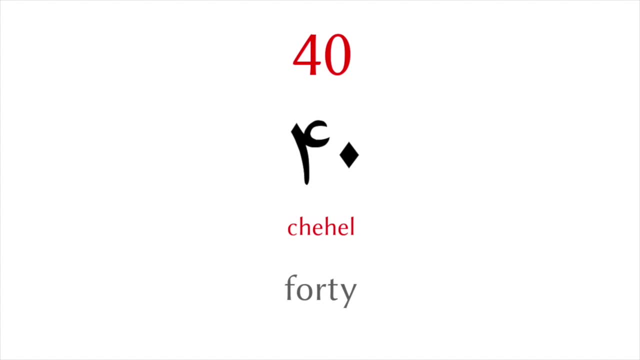 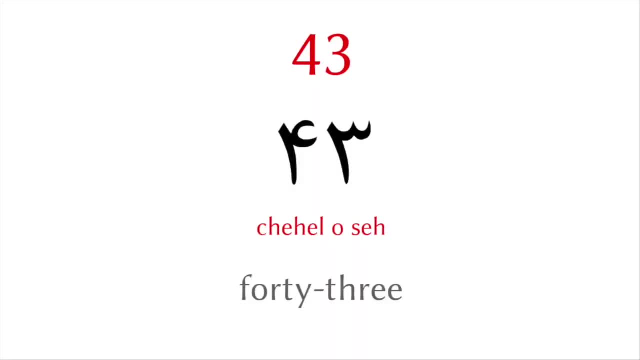 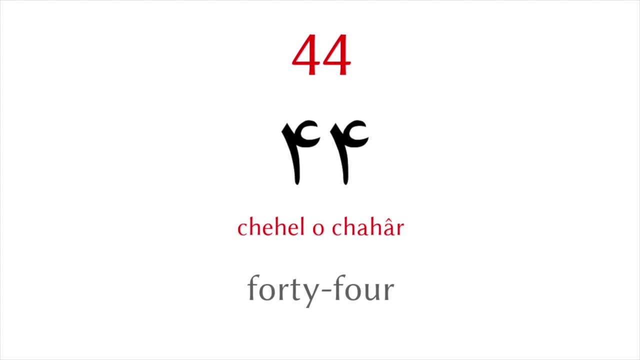 چهلو چهار, Forty-five, چهلو پانج, چهلو پانج, چهلو پانج, Forty-six, چهلو شیش. چهلو شیش چهلو شیش Forty-seven چهلو های چهلو های چهلو های Forty-eight چهلو هاشت. 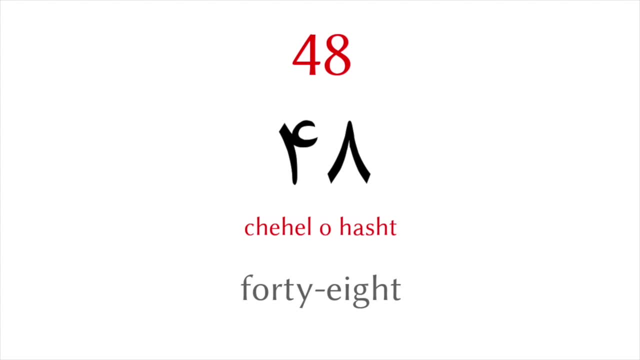 چهلو هاشت, چهلو هاشت Forty-nine Chahelonno, Chahelonno, Chahelonno Fifty, Panjah, Panjah, Panjah Fifty-one. 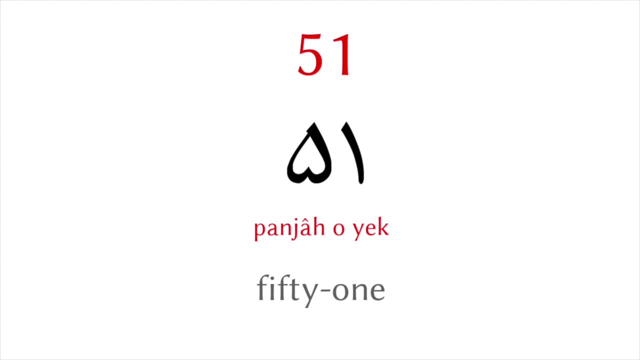 Panjah-o-yek, Panjah-o-yek, Panjah-o-yek. Fifty-two, Panjah-o-do, Panjah-o-do, Panjah-o-do, Fifty-three, Panjah-o-seh, Panjah-o-seh. 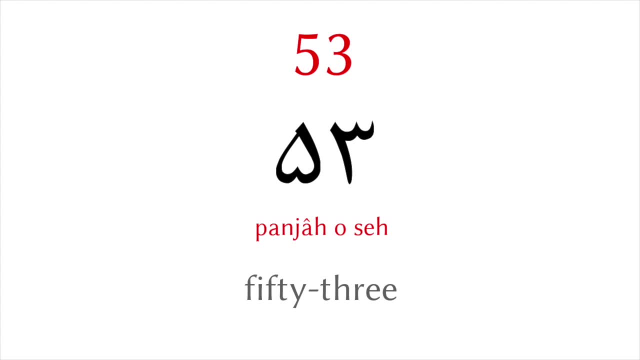 Panjah-o-seh. Fifty-four, Panjah-o-chahar, Panjah-o-cha-haar, Panjah-o-chahar, Fifty-five, Panjah-o-panjh, Panjah-o-panjh, Panjah-o-panjh. 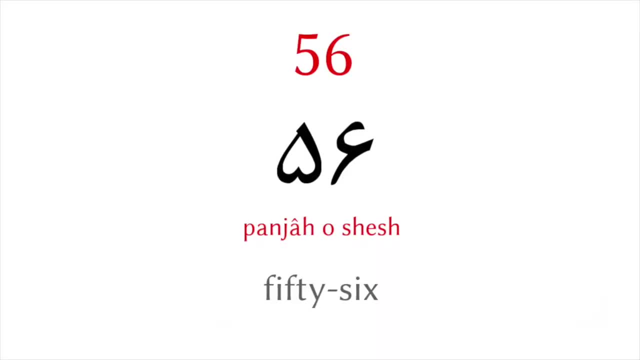 Fifty-six, FIFTY-SEVEN, FIFTY-SEVEN, FIFTY-SEVEN, FIFTY-SEVEN, FIFTY-EIGHT, FIFTY-EIGHT, FIFTY-NINE, FIFTY-NINE, FIFTY-NINE. 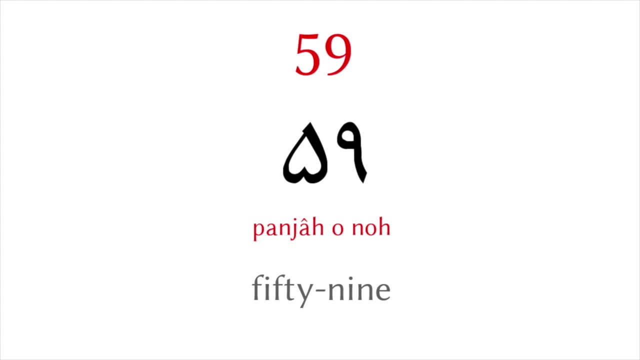 ۵۹۹, Sixty ۶۶, ۶۶, Sixty-one ۶۶, ۶۶, Sixty-two ۶۶, Sixty-three ۶۶, ۶۶. 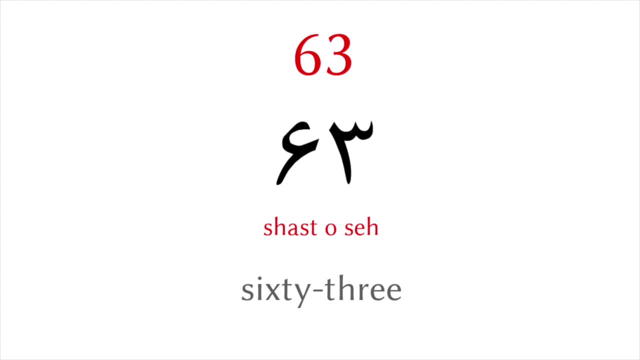 ۶۶. Sixty-four, ۶۴, ۶۴, ۶۴. Sixty-five, ۶۵, ۶۵, ۶۵. Sixty-six, ۶۶, ۶۶. 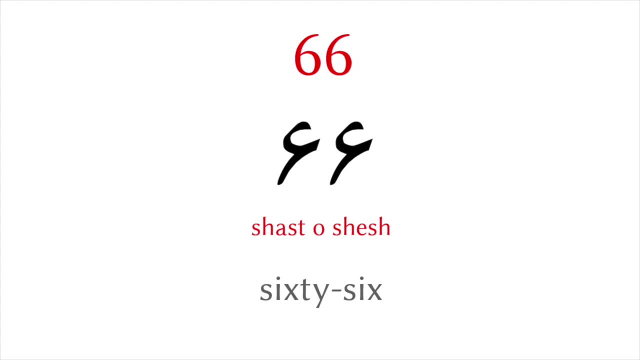 Sixty-six, Sixty-seven, ۶۷, ۶۷, ۶۷, Sixty-eight ۶۸, Sixty-eight ۶۸, ۶۸, Sixty-nine ۶۹, ۶۹. 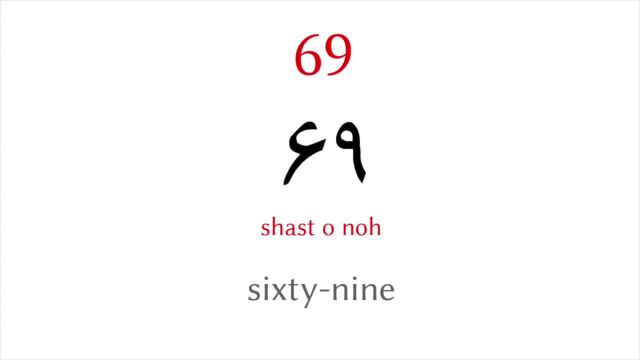 ۶۹, ۶۹, ۶۹, ۶۹, ۶۹. Seventy ۷۰, Seventy-one, Seventy-one, Seventy-two, Seventy-three, Seventy-four, Seventy-four, Seventy-five. 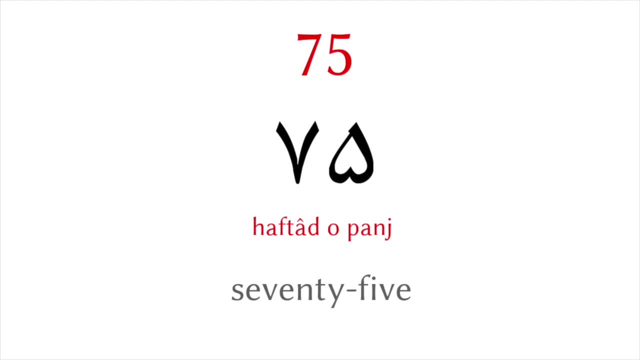 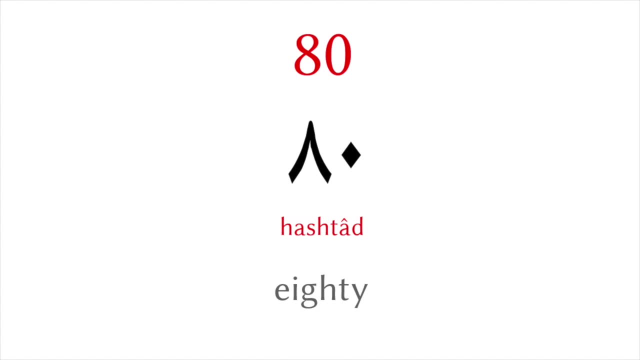 Eighty, Eighty, Eighty, Eighty, Eighty-one, Eighty-one, Eighty-two, Eighty-two, Eighty-two, Eighty-three, Eighty-three, Eighty-three, Eighty-three, Eighty-three, Eighty-three. 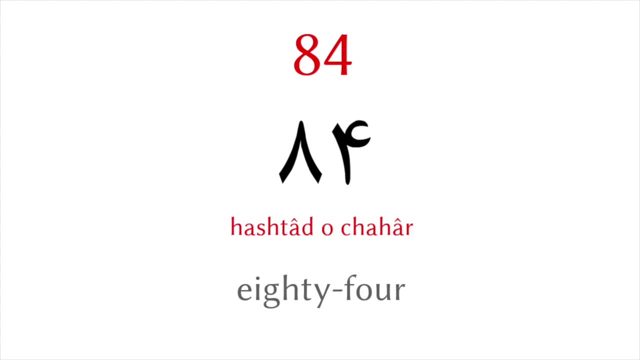 Eighty-four: Haštādo chahār, Haštādo chahār, Haštādo chahār. Eighty-five: Haštādo panj, Haštādo panj, Haštādo panj. 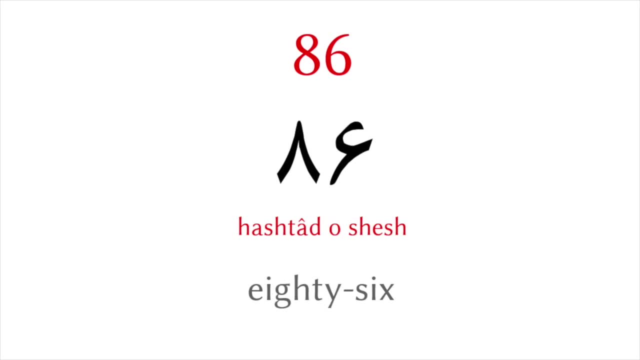 Eighty-six Haštādo shesh, Haštādo shesh, Haštādo shesh. Eighty-seven. Haštādo haft. Haštādo haft, Haštādo haft Eighty-eight. 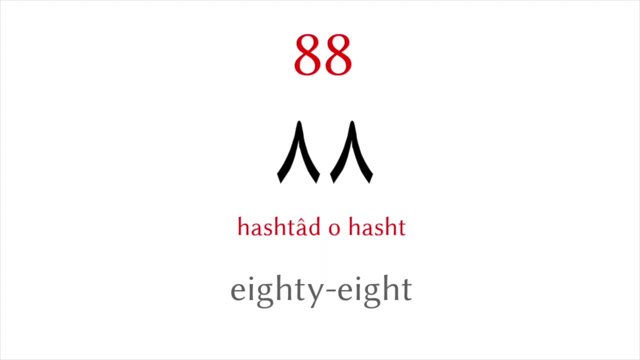 Haštādo hašt Haštādo hašt Haštādo hašt Eighty-nine Haštādo no Haštādo no Haštādo no Ninety Navad Navad. 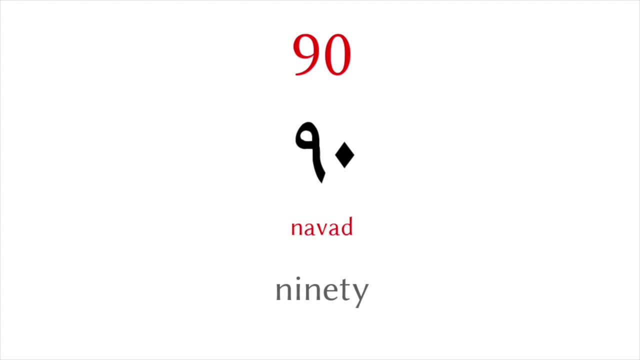 Navad. Ninety-one, Ninety-two, Ninety-three, Ninety-four, Ninety-four, Ninety-five, Ninety-six, Ninety-six, Ninety-seven, Ninety-seven, Ninety-eight, Ninety-eight, Ninety-nine, Ninety-nine, Ninety-nine, Ninety-nine. 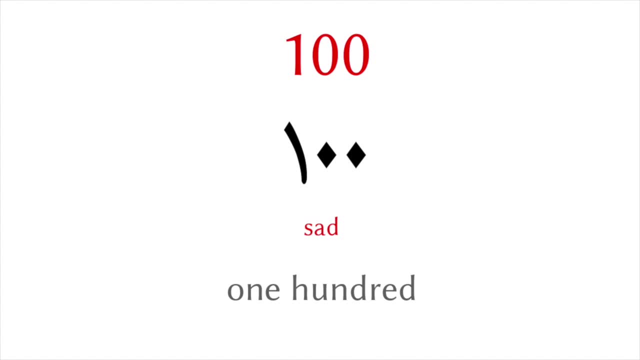 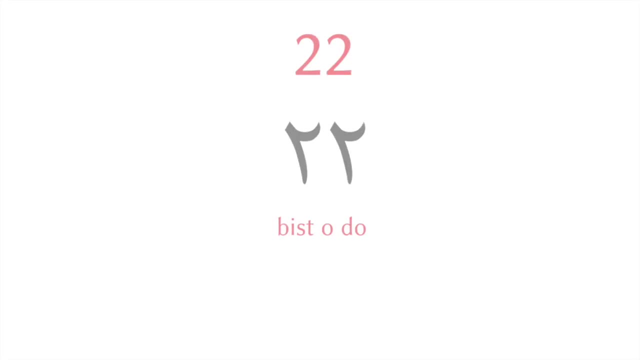 21,, 22,, 23,, 24,, 25,, 26,, 27,, 28,, 29,, 30, 31,, 32,, 33, 33,, 34,, 35,, 36,, 37,, 38,, 39,, 40. 41,, 42,, 43,, 44, 45, 46, 47, 48, 49, 50, 51, 52, 53, 54, 55, 56, 57, 58, 59, 60, 61, 62, 63, 64. 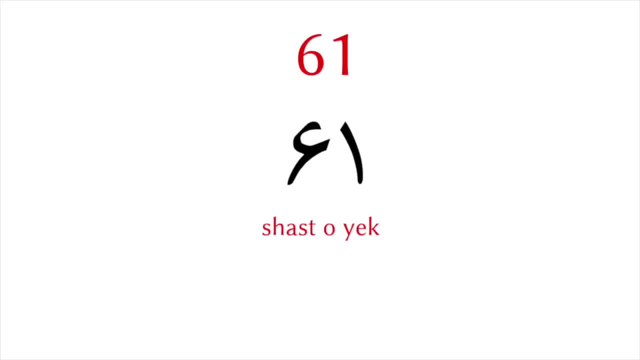 65, 66, 67, 68, 69, 70, 70, 71, 72, 73, 73, 74, 75, 76, 76, 77, 78, 79, 80, 81, 82, 83, 68, 69, 72, 71. 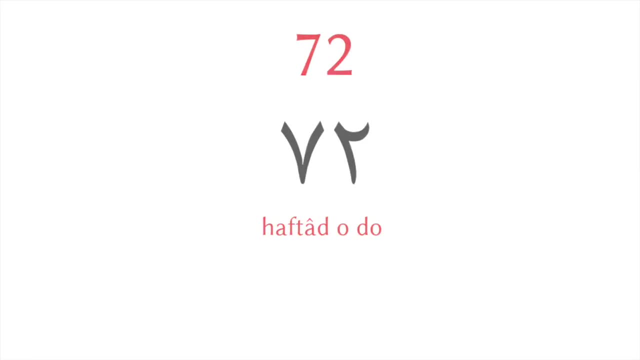 72, 72, 72, 72, 72, 73, 72, 73, 74, 74, 74, 75, 75, 76, 76, 77, 77, 76, 77, 77, 77, 77, 88, 88, 89, 89.